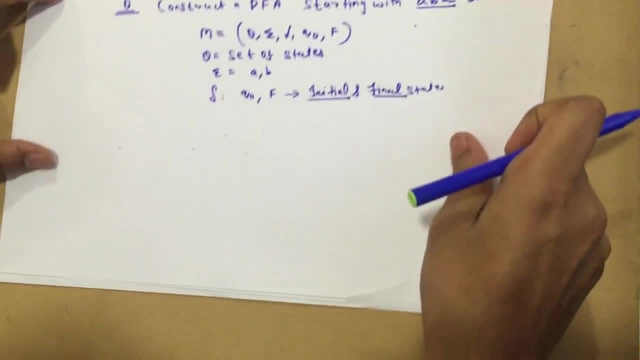 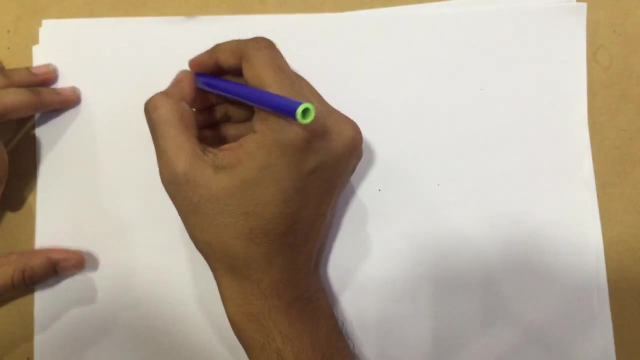 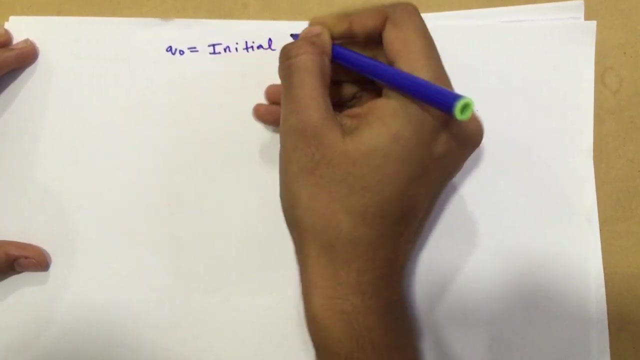 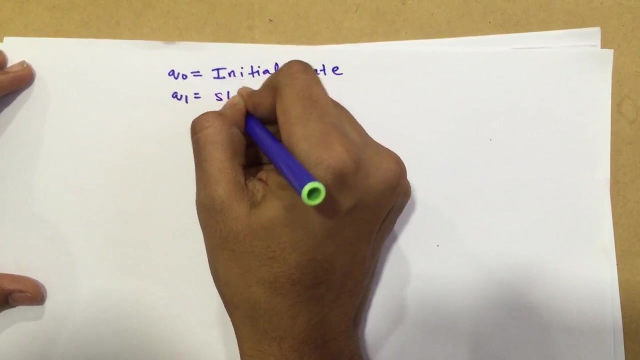 should go to the final state. So how do you do this? Well, we are going to use a very simple approach. First, we are going to declare the states. So initially, obviously Q0 will be my initial state, because that's where I start off. Q1 is the state which is starting with A. So remember, we have to find 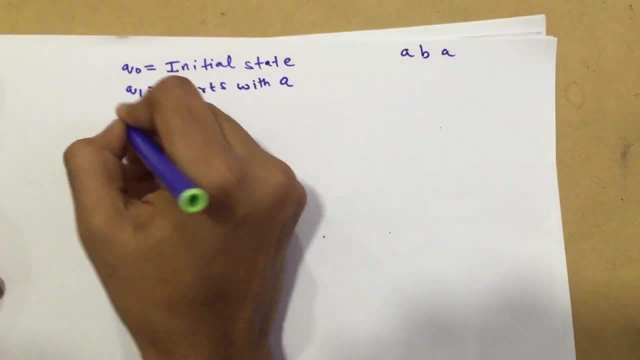 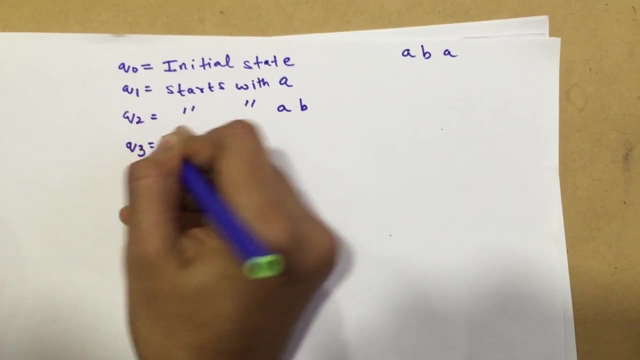 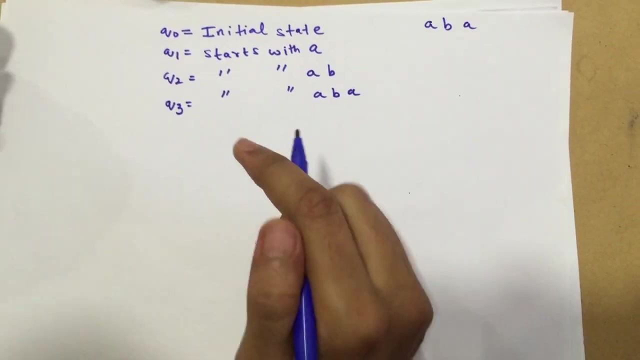 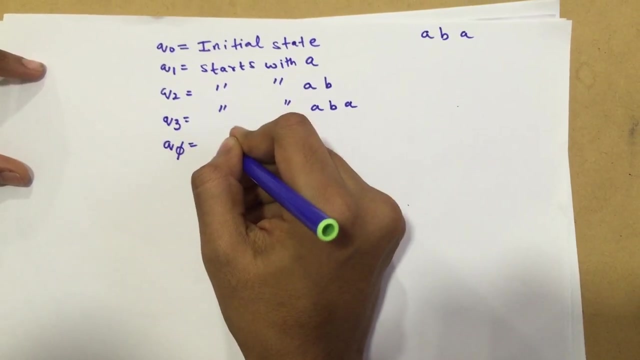 a DFA for strings starting with ABA, Q2 will be a state which starts with AB and Q3 is a state which starts with ABA. Also, in this problem, the only difference from the last problem where we did with the ending was is we take a null state, Q5, where, if the string is not starting with ABA, we will put. 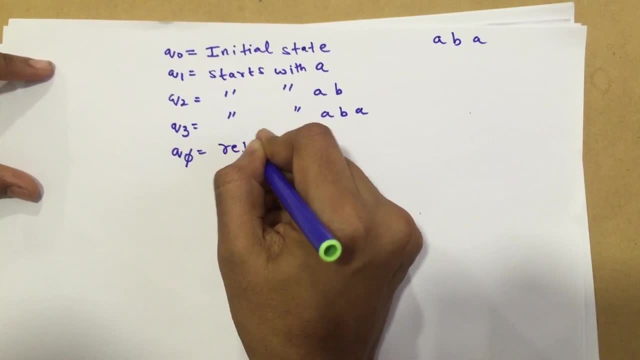 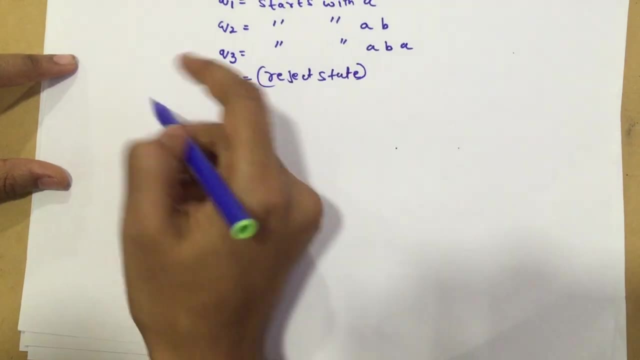 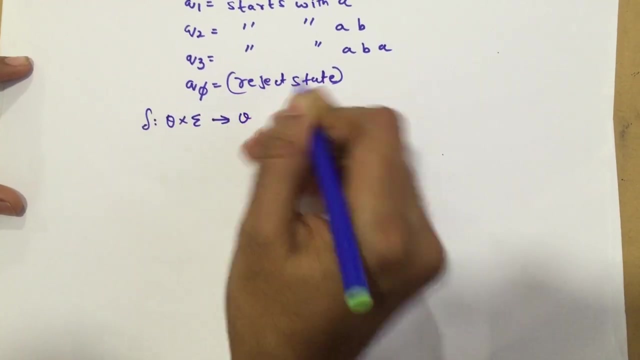 the string in this state. This is also called my reject state. Okay, So I said I am going to explain to you guys what this function was. Well, this function is going to give me Q into summation. gives me Q, So I am going to draw a Q versus summation. 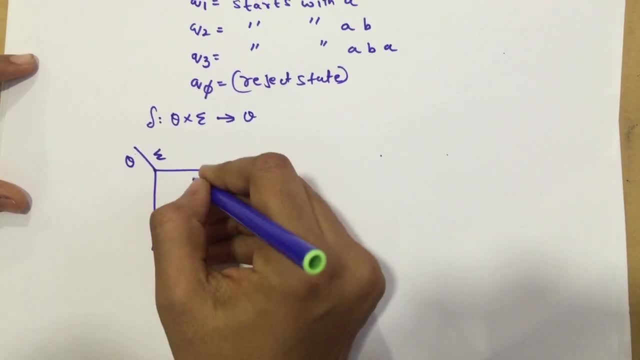 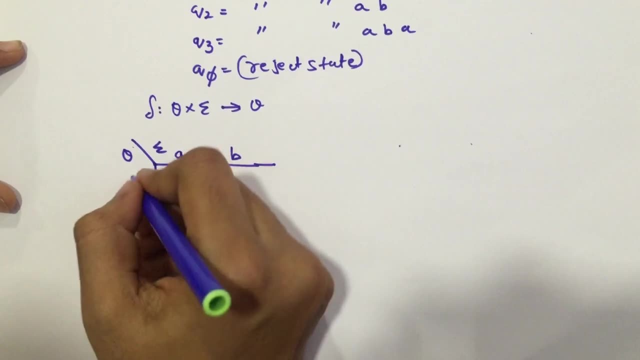 table and it is going to give me the results are going to be of Q only, So it will be the Q0, Q1, Q2, Q3 or the Q5.. So I am going to write here: Q0,, Q1, Q3, Q4,, Q5,, Q6, Q7, Q8, Q9,, Q10,, Q11,, Q12,, Q12,, Q13,, Q13,. 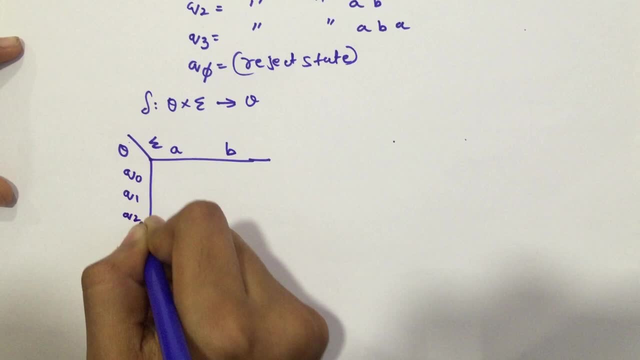 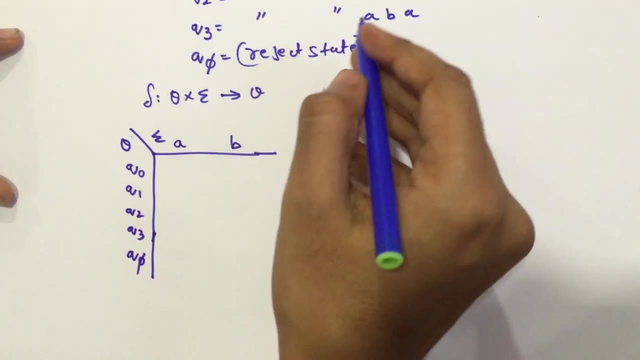 Q14, Q14, Q15, Q16, Q17,, Q18,, Q19,, Q20,, Q21, Q21,, Q22,, Q23 and Q15.. So, just for convenience, let us just mention what. so this was my initial state, or I can call it epsilon, and this was: 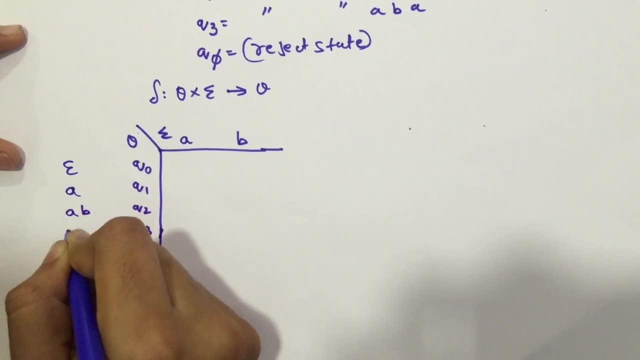 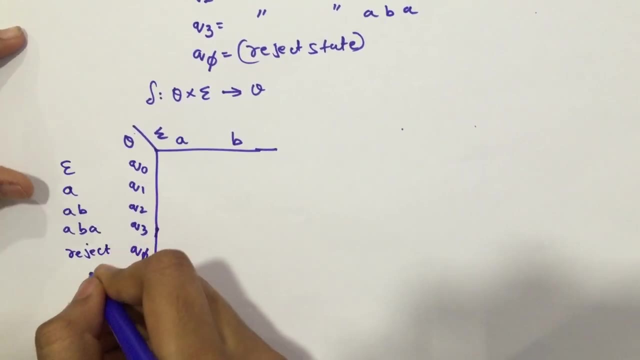 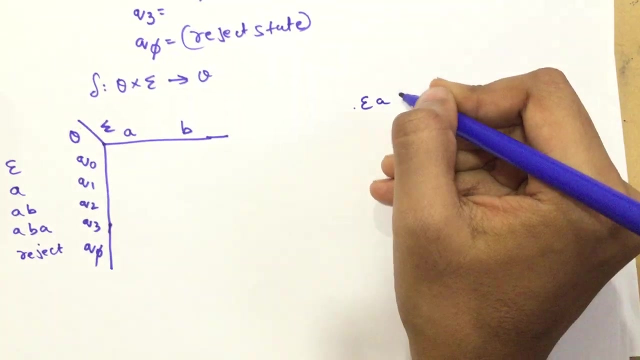 my string starting with A string starting with AB string starting with ABA, and it was my reject state. So the strings which do not start with ABA go here. So if I put A with epsilon, I get epsilon A, So that is effectively equal to A. So since 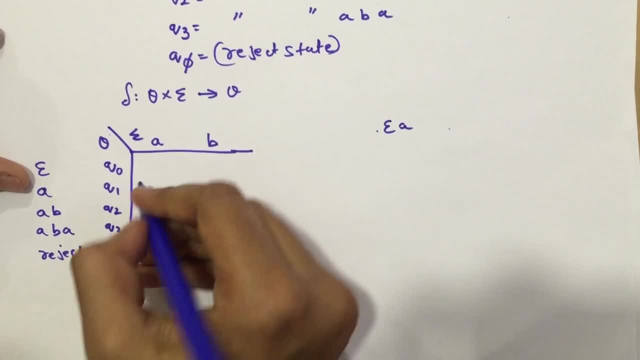 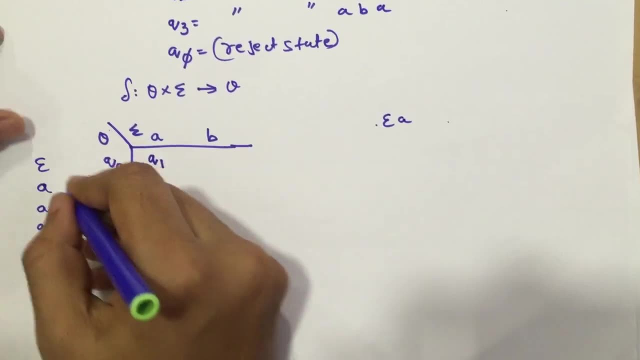 Q1 says that this Q1 is the state which starts with A. we are going to put Q1 here. Now let us take B Does B. can we find B anywhere here? So no, B does, the string does not start. 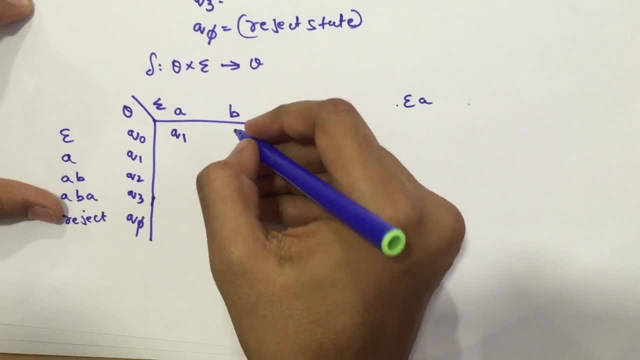 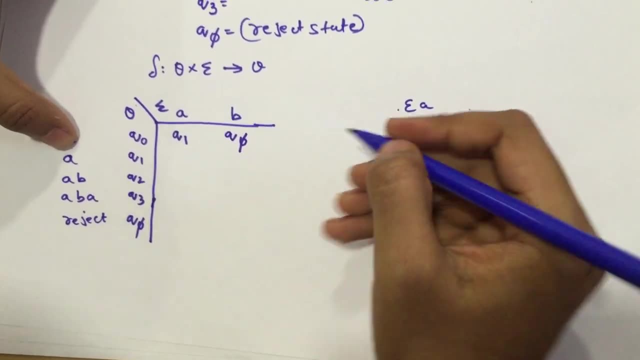 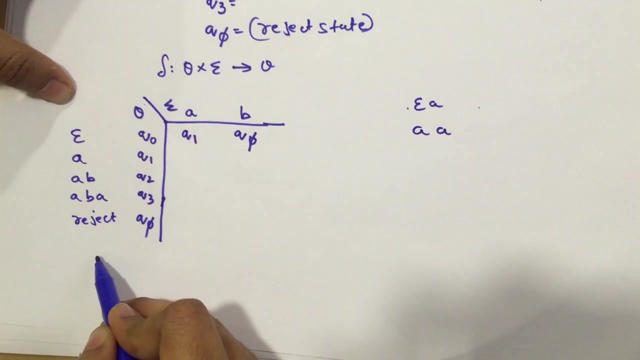 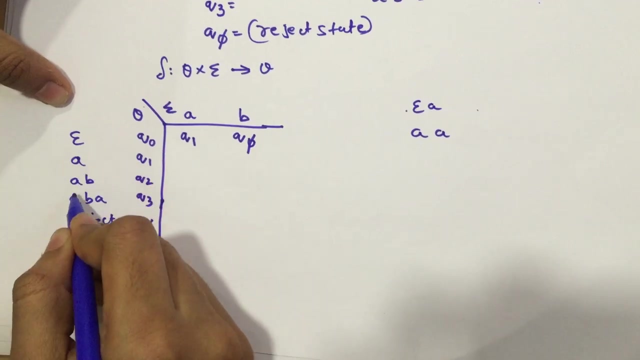 with A or AB or ABA. So we directly put it into the reject state, That is, Q5.. Now we take the next state, which is Q1, A. So when Q1 goes with A, I get AA. So can I find anywhere here AA? No, So does it start with ABA? does it start with A? does? 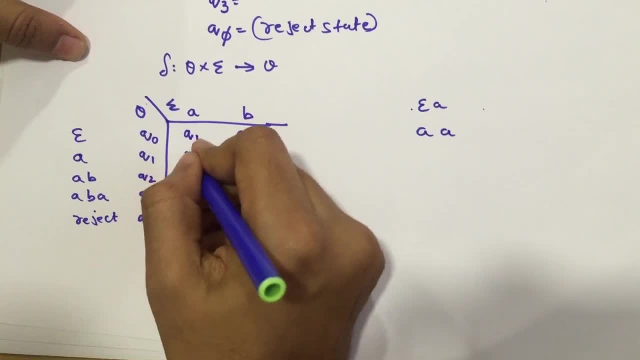 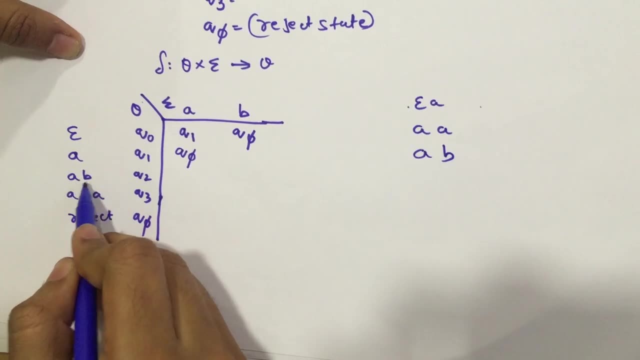 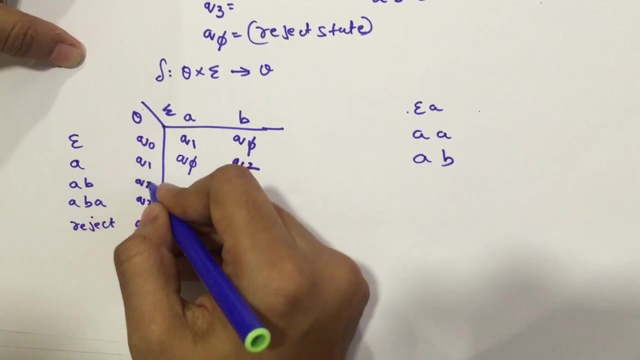 it start with AB. does it start with ABA? No, So I directly reject it. Now I am going to take AB. So do I have a state where it starts with AB? Yes, So I am going to put it into Q2.. Now let us take Q2, that is AB, Q2 when combined. 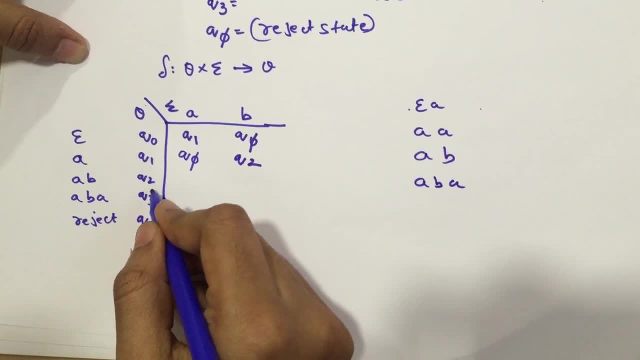 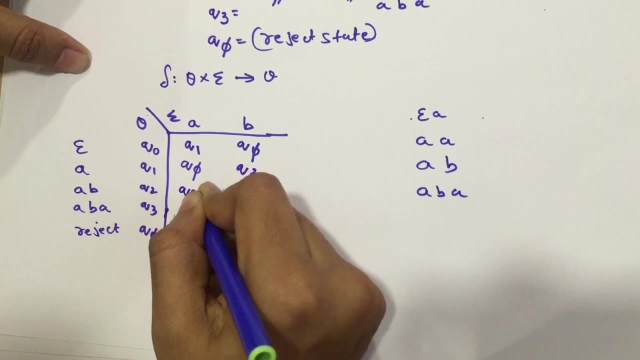 with A, I get ABA. So do I have a state that says I have a string starting with AB? Yes, I do. So that state is Q3, since Q3 is starting with ABA, So I am going to put Q3 here Now. 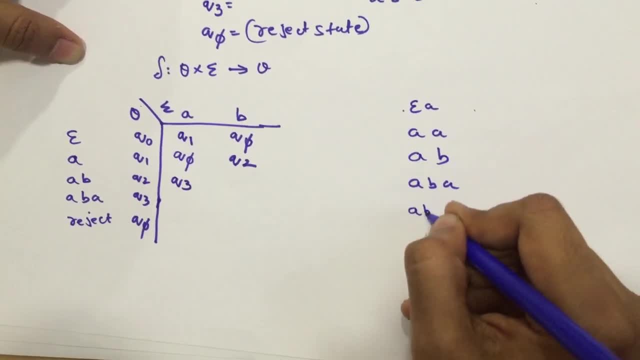 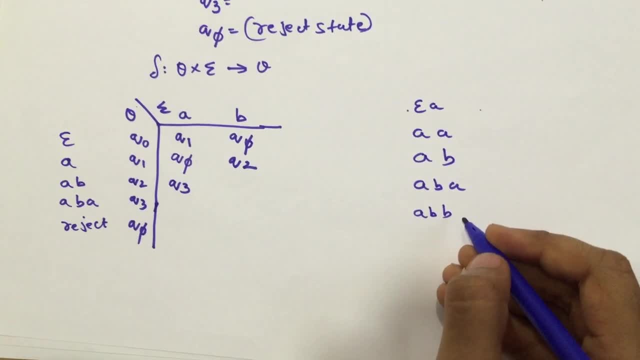 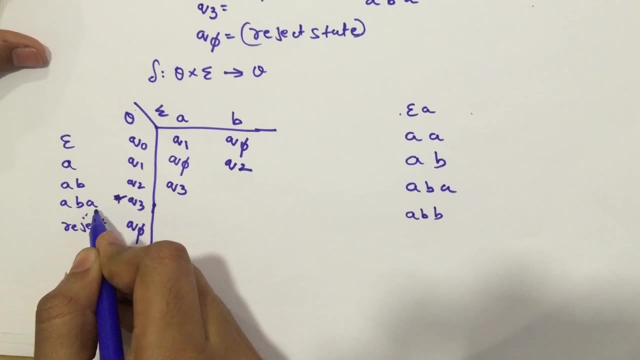 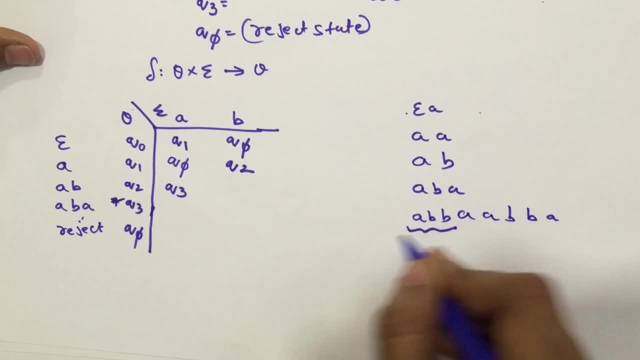 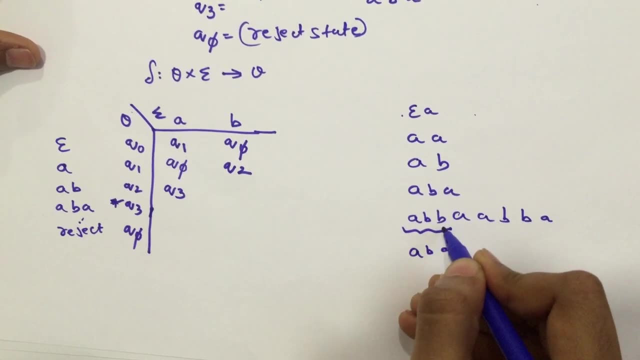 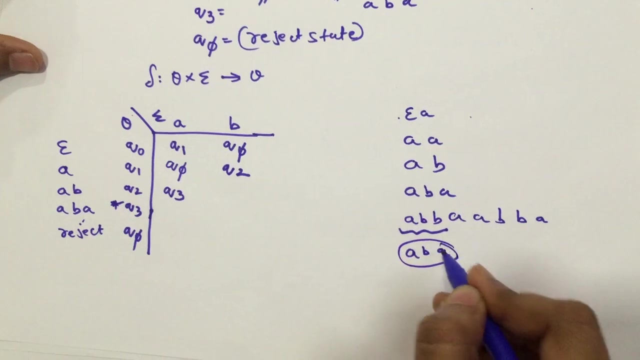 my starting will always remain ABB. No way I can change this to ABA, can I? So hence, if you have a doubt that, although ABB is, I cannot find ABB here. but this string will starts with a, b, but it will never reach the final state, which is a, b, a. so we directly. 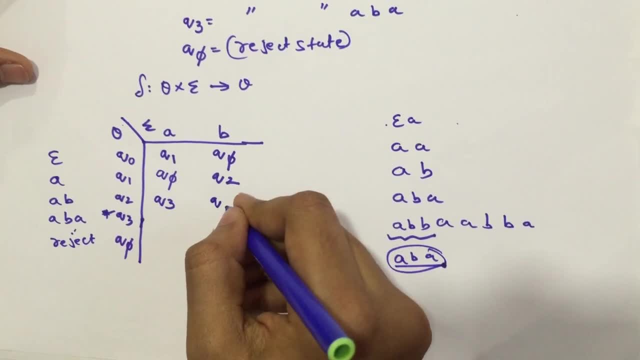 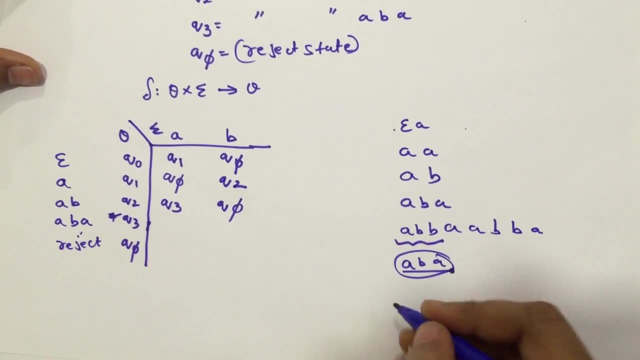 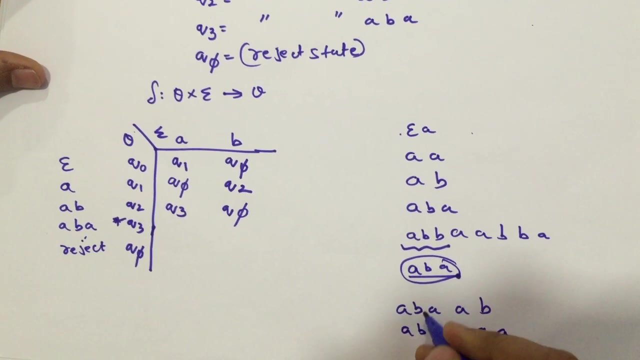 put this string into reject. so hence we reject this q file. so now we have q3, which is starting with a, b, a. now if I put any letters, let's say a, b, a, I put a, a, I put a, b. or let's say I put a, b first and then an a or a, it will always start with a, b, a, always, no matter what, 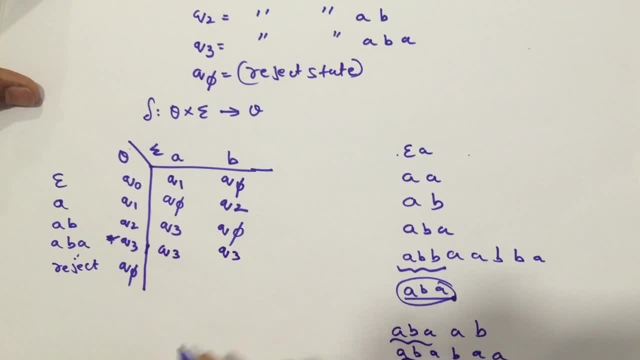 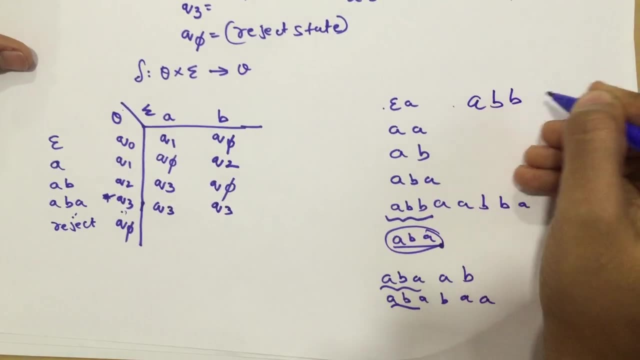 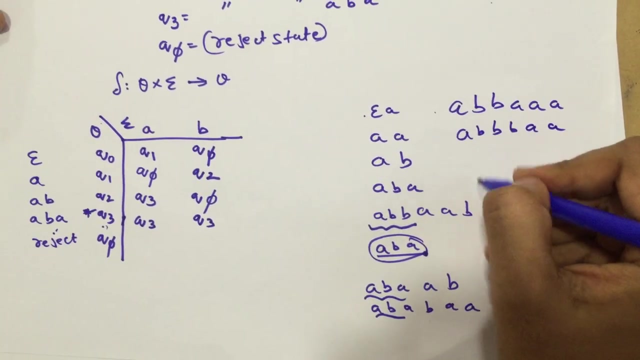 happens. so this stays in my q3 itself. and then if my, if my string is already rejected- let's say it starts with a b b instead of a b a- and if I add any letters, any damn letters okay, which are defined in the input, my string will always remain rejected because it never. 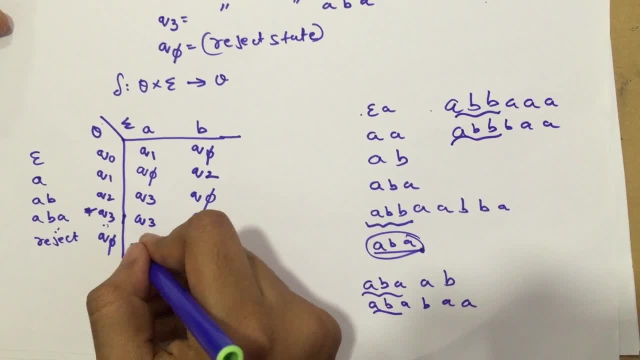 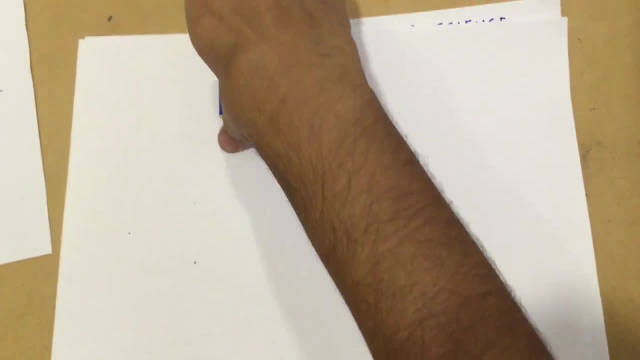 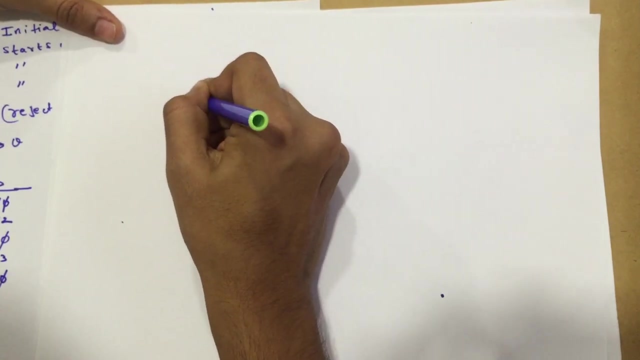 started off with a, b, a in the first place, so hence I'm going to put a q file here and a q file here again. so now let's draw the transition diagram for the same, and we're going to do this using these states only. okay, so first I'm going to draw a q0 here, and on the input of a, when 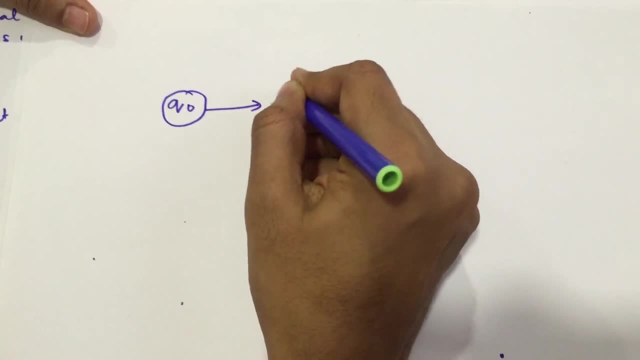 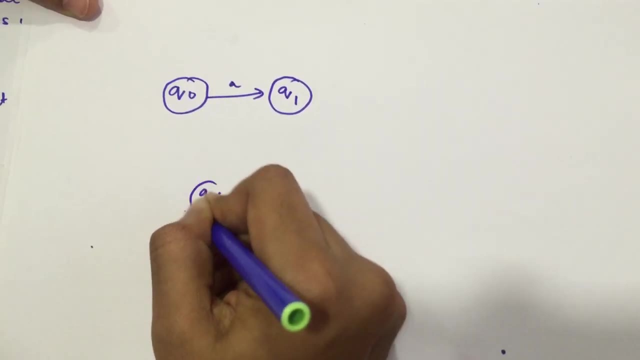 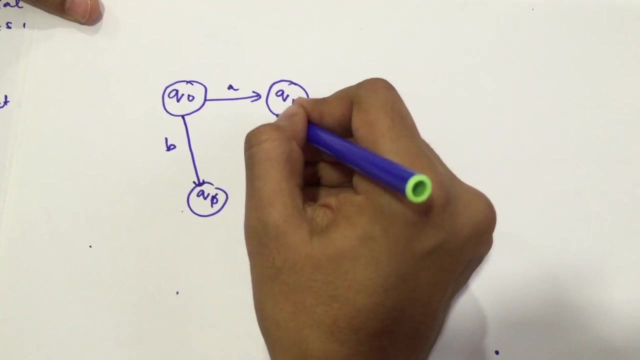 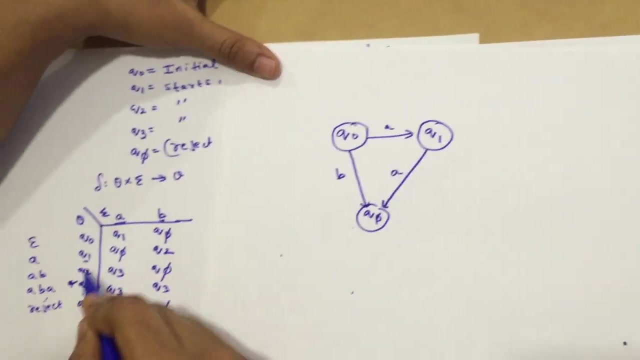 I get, so I click: I go to q1. now, when I get a b, I put it into reject state on q1. when I get a b, I put it into q5. I'm looking only in the diagram on q1. when I get a b, I go to. 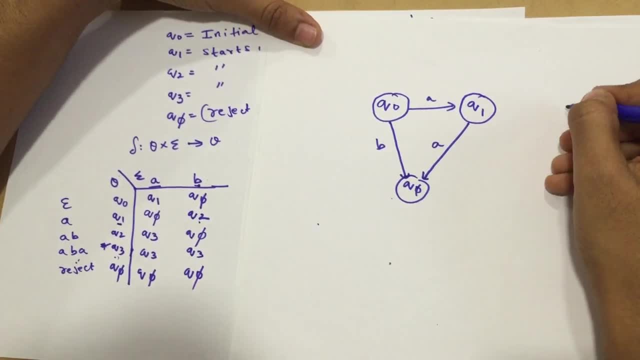 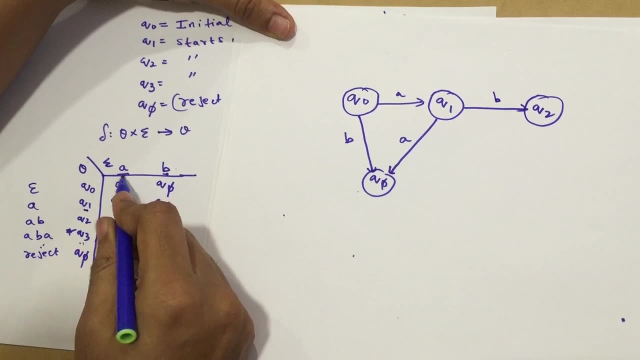 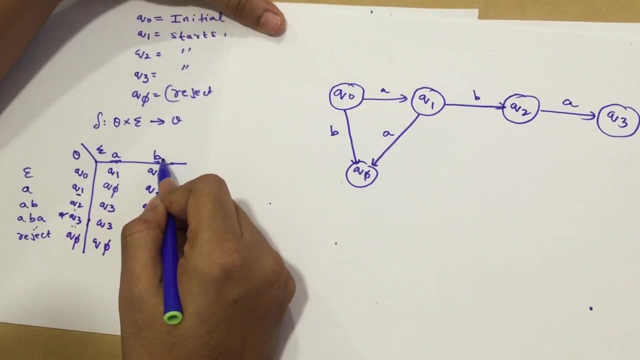 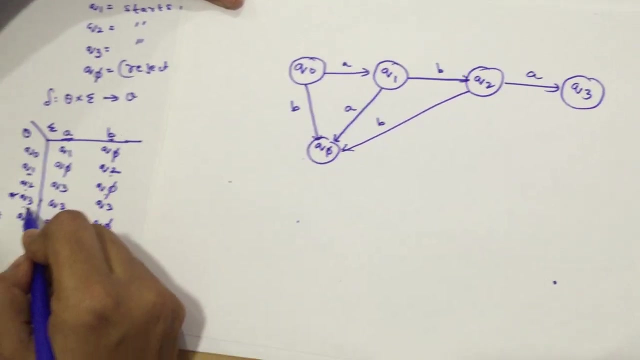 q2. so let's make a q2 and this goes to b. on q2, when I get an a, I go to q3. on q2, when my input is b, it goes to q5.. on Q3, when my input is A, it goes to Q3 itself. 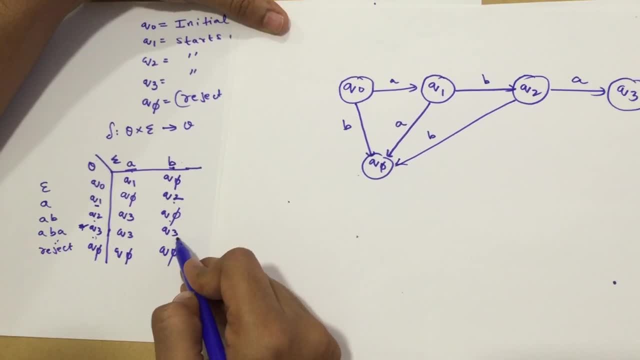 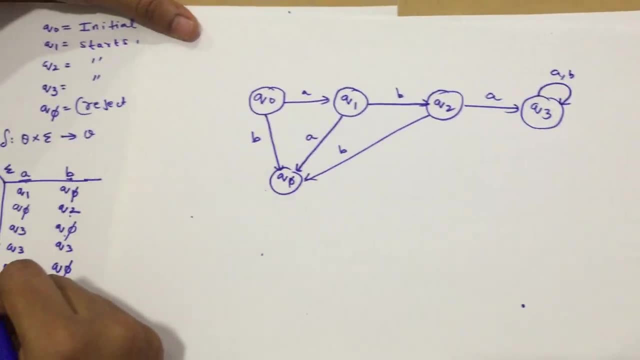 and on Q3. when my input is B, it goes to Q3 itself again. so I'm gonna make a self loop here with A, B and on Q5. when I put A, it remains in my reject state, and when on Q5 I put B, it also remains in my reject state.